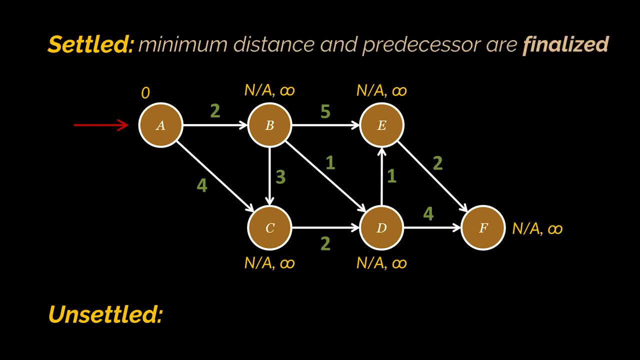 Settled nodes are the ones with a known minimum distance from our source, the ones where the minimum distance and the predecessor are filled and finalized. The unsettled nodes are the nodes we can reach from the source, but we still don't know the minimum distance phảir of our source, because we don't know theitters and 설�blueink and fillerns from the sources. but instead of these, of course, we have the nodes located at both the citizens and the universal nodes which we can easily reach from the group. 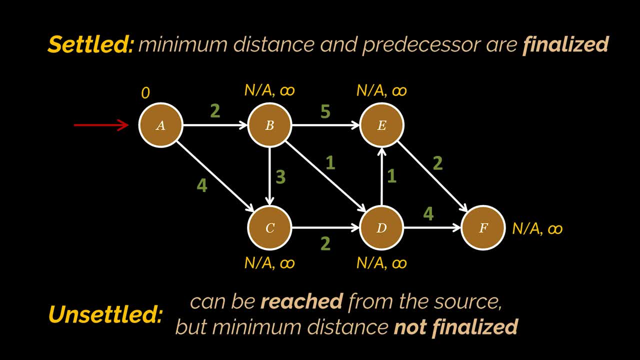 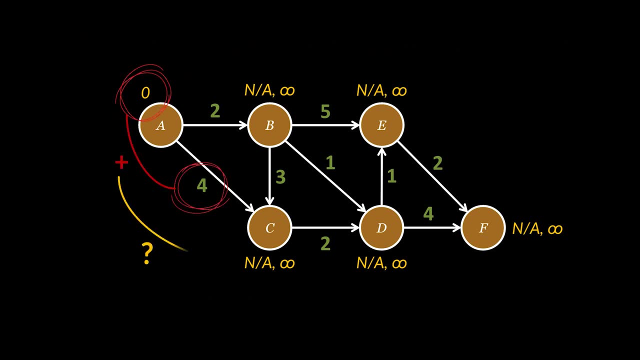 general, that separates them from that source node. Okay, the first thing we need to do is pick the node with the lowest known distance and then evaluate all its unsettled adjacent nodes. The idea is to add the edge weight that separates our source from its adjacent node. 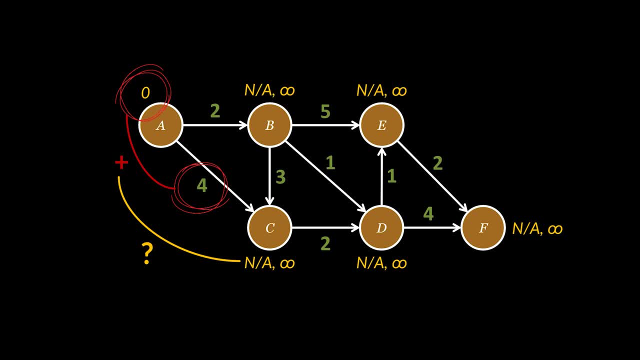 to the source distance, then compare it to the destination's distance. Example: for node B, 0 plus 2 is lower than infinity. So the new distance for node B is 2, and the new predecessor is A. The same applies to node C. 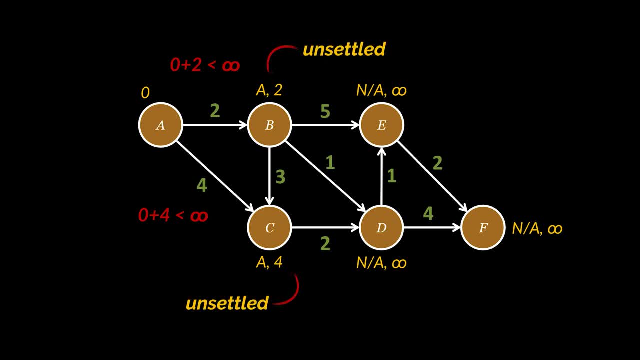 Node A is now considered settled. Nodes B and C are added to the unsettled nodes because they can be reached from the source, but we still need to process their adjacent nodes and make sure that the distances we picked are indeed the minimum. Now that we have two nodes in the unsettled set. 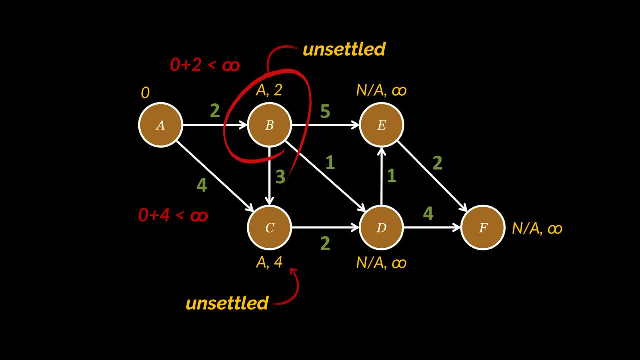 we choose the one with the lowest distance, in this case node B. then we reiterate the same process until we settle all nodes in the graph. So next we check the adjacent nodes of B. Let's take C And, as you can see, the edge weight from B to C. 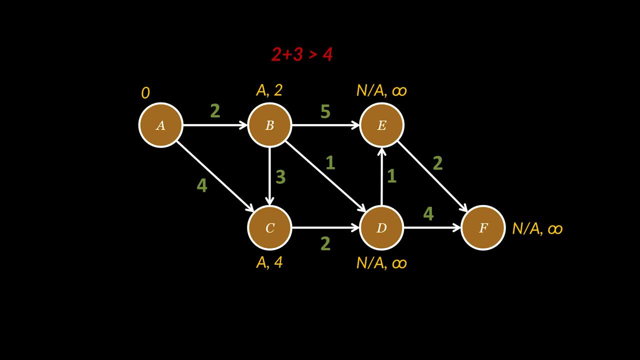 added to the minimum distance of B is bigger than the previously evaluated distance of C. Therefore, the distance of C we had is indeed the minimum. After repeating this process on all the available nodes, we will be able to calculate the minimum distance and path from A to all of the graph nodes. 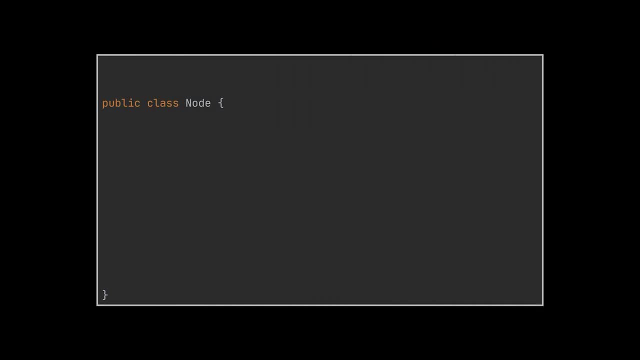 Ok, let's go ahead and try to implement this algorithm, and I guarantee after this, things will be way clearer. To find the optimal path between the nodes of a graph, we actually need nodes or vertices, So the first class we are going to create is the node class. 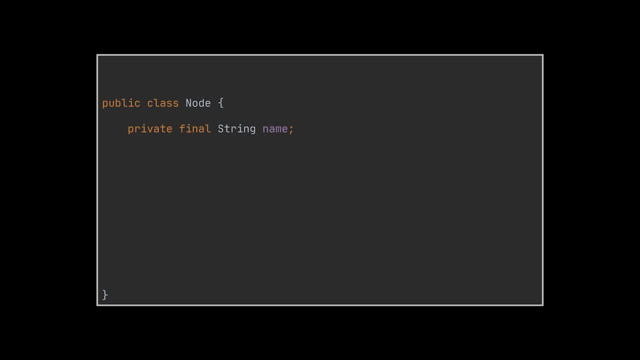 This one will house the name of the node in our example, A, B, C, etc. The minimum distance of that node which starts off as the integer dot max value in order to simulate infinity A map storing the adjacent nodes of that node. 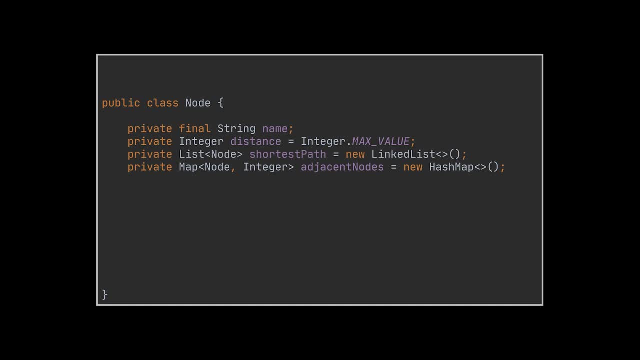 and the edge weight separating them. And, finally, a list storing the shortest path from the source node, which will be later updated by the Dijkstra algorithm. To help us with the implementation, I added two helper methods: The addAdjacentNode method. 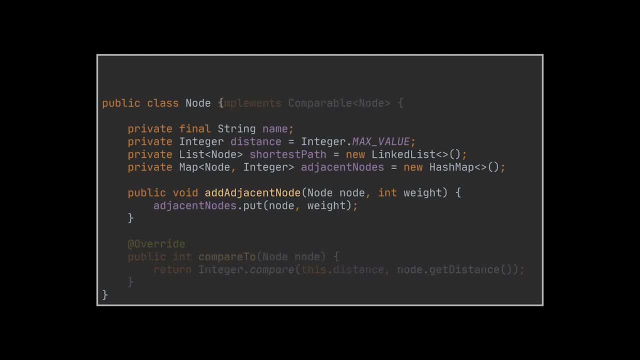 which takes a node and the edge weight separating them, And I overwrote the compareTo method. This was done because we will be making use of a priority queue to poll the unsettled node with the smallest distance. So we are going to use the Dijkstra algorithm to set the distance of the source node we picked to zero. 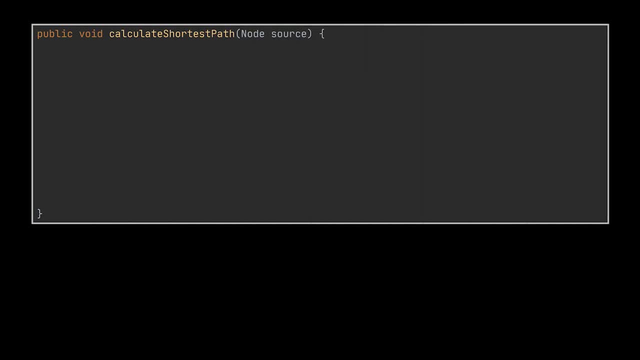 We are going to use the Dijkstra algorithm to set the distance of the source node we picked to zero. Next, we are going to create the settled and unsettled sets we talked about. The unsettled set will actually be the priority queue and the source node will be added to it right from the start. 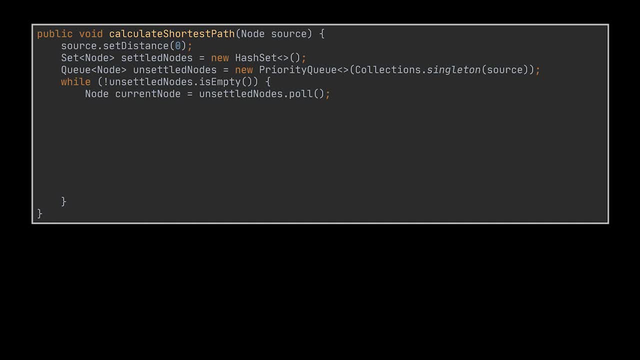 So, while this queue is not empty, what we are going to do is poll the node with the minimum distance from it, And then we are going to loop over its adjacent nodes More precisely, for each adjacent node that isn't settled, meaning we still don't have a decisive minimum distance for it. 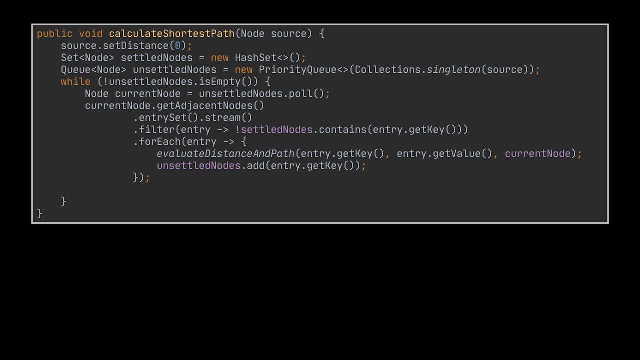 we are going to update that node's distance and shortest path via the evaluateDistanceAndPath method, which we will be implementing in a sec, And then we will insert this node in the queue of unsettled nodes After we loop over all of the nodes. adjacent nodes we polled. 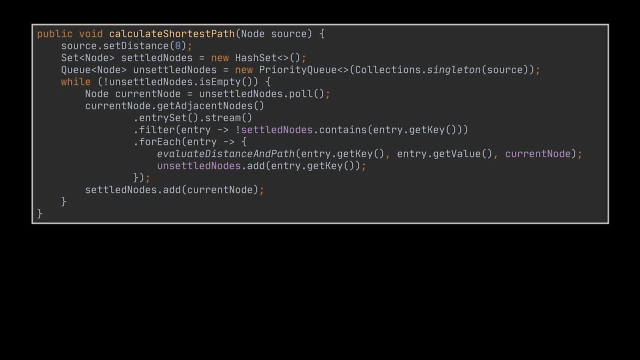 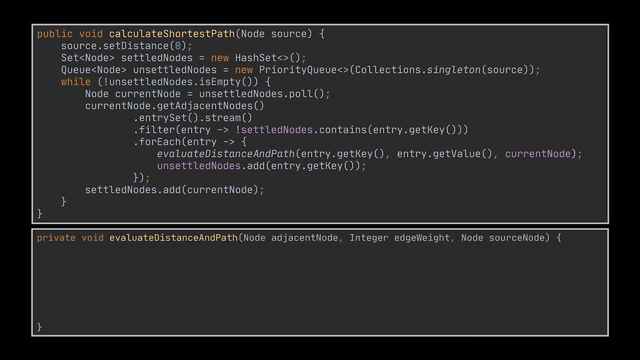 we add the node- the one we are currently working with- to the set of settled nodes. Okay, let's take a look now at this evaluateDistanceAndPath helper method we made use of inside the for loop. We previously mentioned that we need to compare the sum of the edge weight. 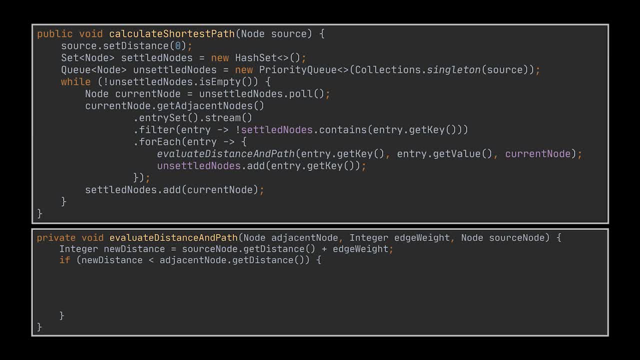 and the distance of the source node. it connects to the destination's distance, And that is exactly what we are doing here Now. if the distance calculated is smaller than this and that of the node we are trying to reach, then we found a smaller, a more optimal path linking this node to the source.